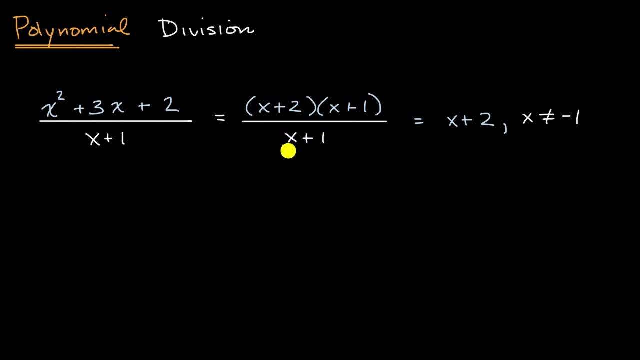 But as we see for any other x, as long as we're not dividing by zero, here this expression is going to be the same thing as x plus two, and that's because x plus two times x plus one is equal to what we have in this numerator here. 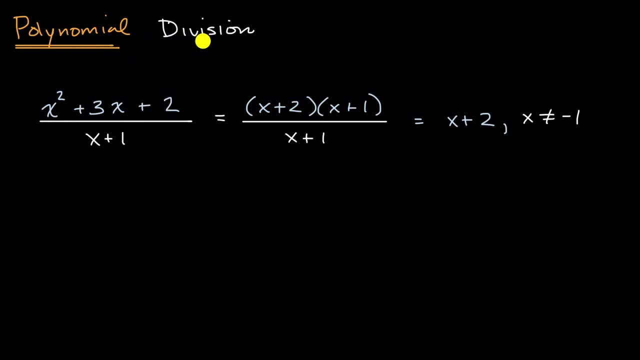 Now, as we go deeper into polynomial division, we're going to approach things that aren't as easy to do just purely through factoring, and that's where we're going to have a technique called polynomial long division. polynomial long division, sometimes known as algebraic long division, 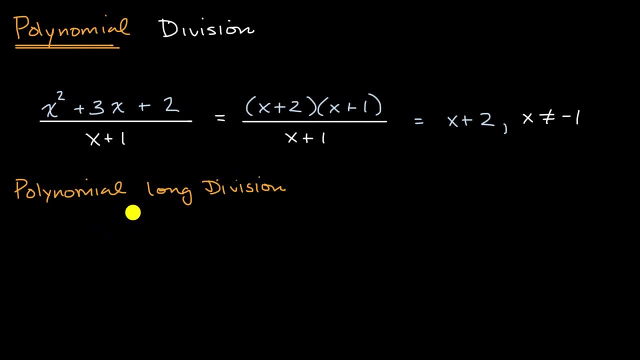 And if it sounds familiar because you first learned about long division in fourth or fifth grade, it's because it's a very similar process, where you would take your x plus one and you would try to divide it into your x squared plus three, x plus two. 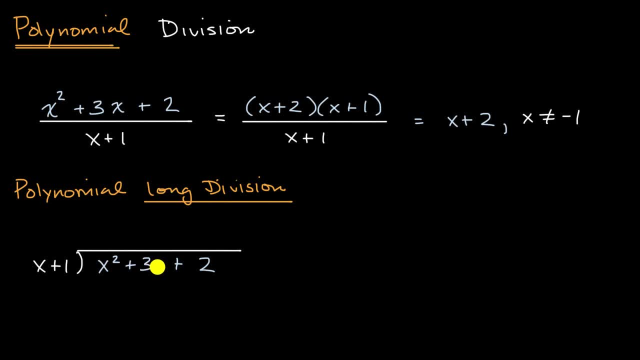 And you do something very- and I'm going to do a very quick example right over here, but we're going to do much more detailed examples in future videos- but you look at the highest degree terms. You say, okay, I have a first degree term. 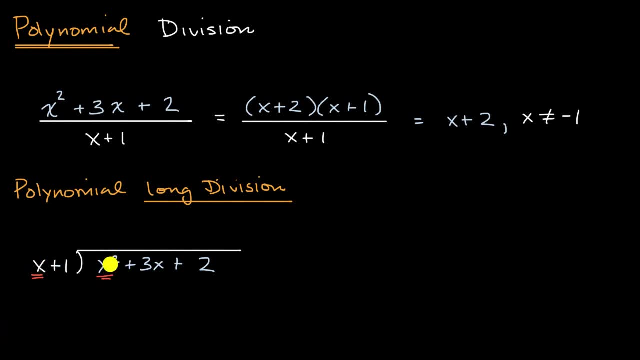 and a second degree term here. How many times does x go into x? How many times does x go into x squared? Well, it goes x times. So you put the x in the first degree column and then you multiply your x times x plus one. 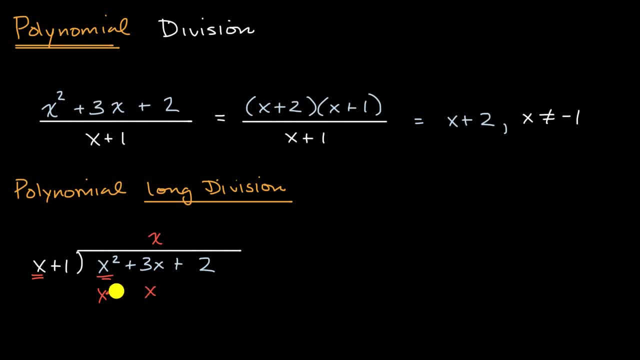 X times x is x. squared X times one is x. And then you subtract this from that, So you might already start to see some parallels with the long division that you first learned in school many years ago. So when you do that, these cancel out. 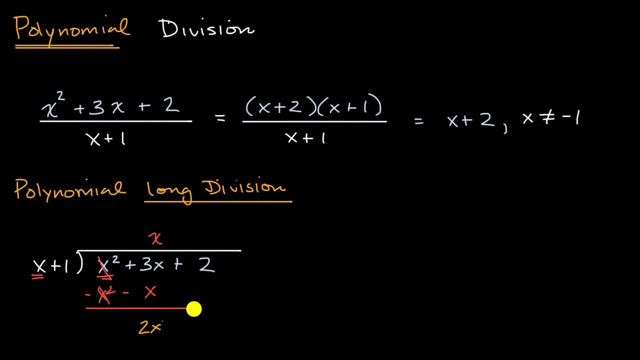 Three x minus x. We are left with a two x, And then you bring down that two, So two x plus two. And you say: how many times does x go into two x? Well, it goes two times, So you have a plus two here. 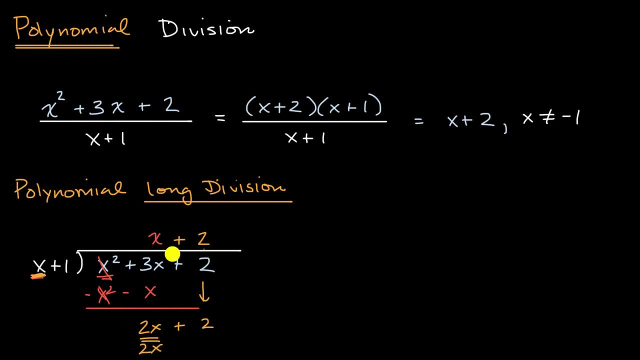 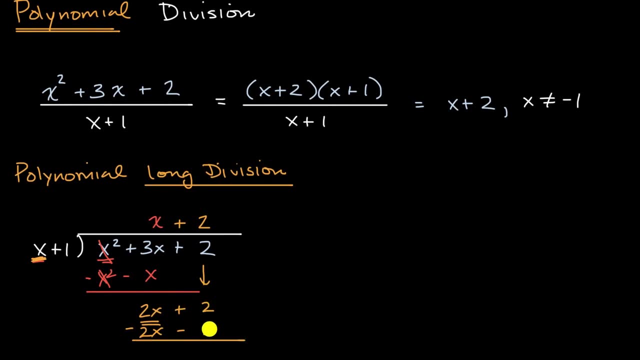 Two times x plus one. Two times x is two x. Two times one is two. You can subtract these And then you are going to be left with nothing. Two minus two is zero. Two x minus two x is zero. So in this situation it divided cleanly into it. 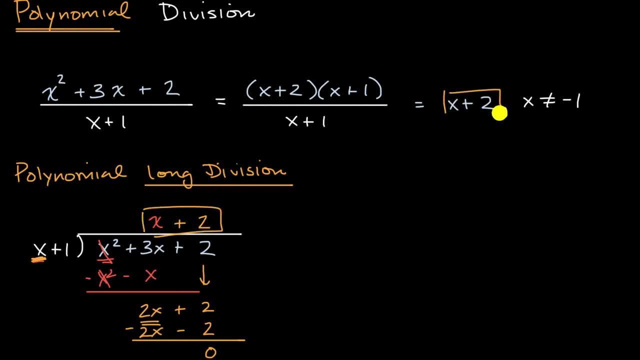 and we got x plus two, which is exactly what we had over there. Now, an interesting scenario that we're also going to approach in the next few videos is what if things don't divide cleanly, For example, if I were to add one.